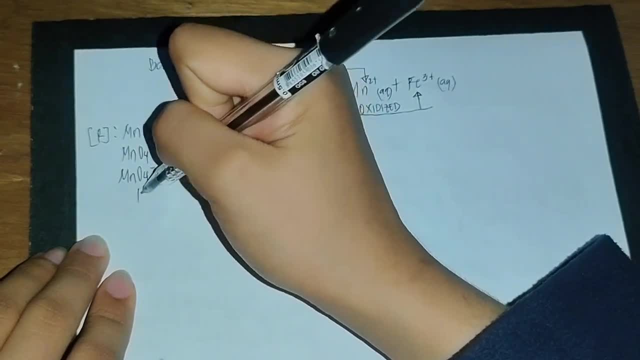 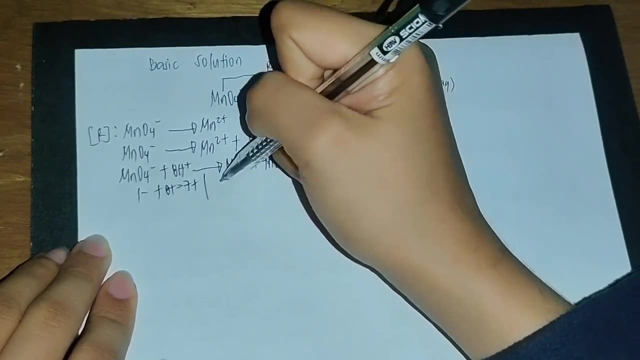 So now we have to balance the charges. We have one negative here plus eight positive equals seven positive. So now we have to balance the charges. We have one negative here plus eight positive equals seven positive, While on the other side we only have two positive. To balance the charges, we need to add a five. 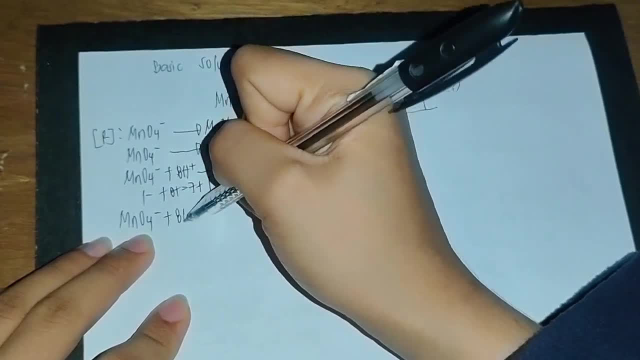 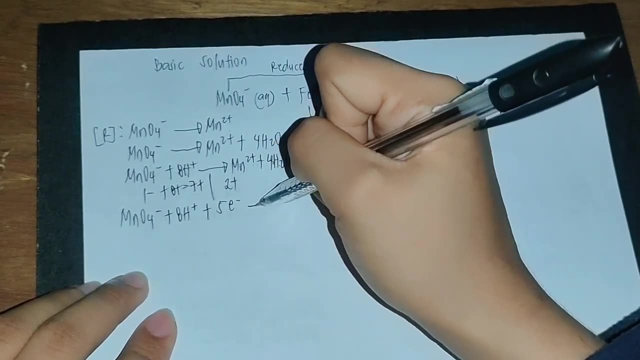 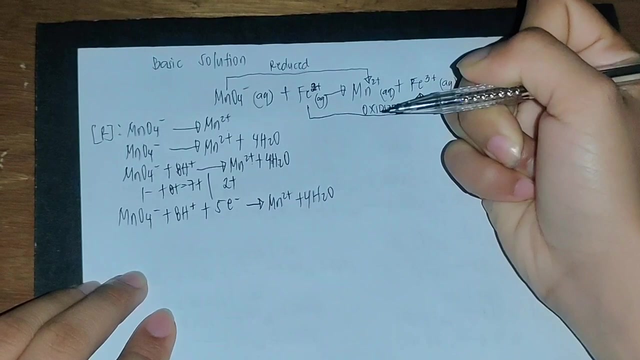 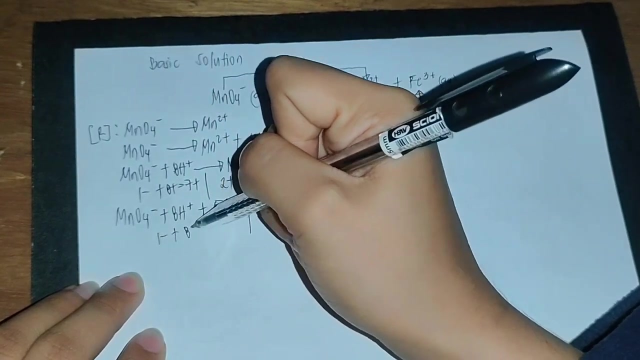 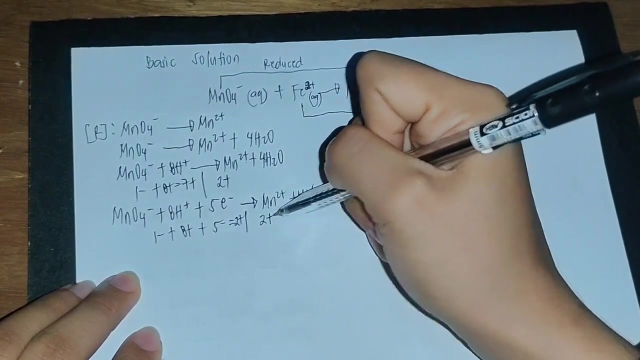 electron here, So MnO4 negative plus H plus plus five electron, and then copy Mn2 plus plus 4H2O. So the charges are: are one negative plus eight positive plus five negative equals two positive, and then we have here two positive. So the charges are now balanced. 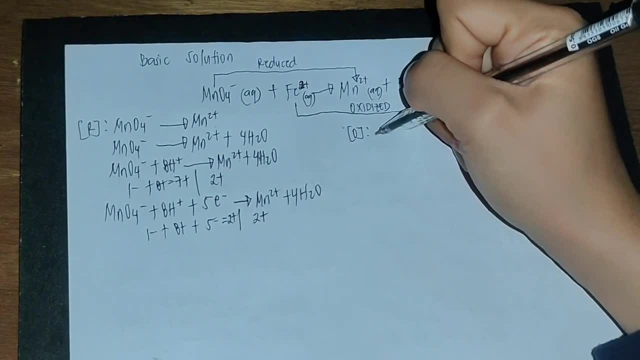 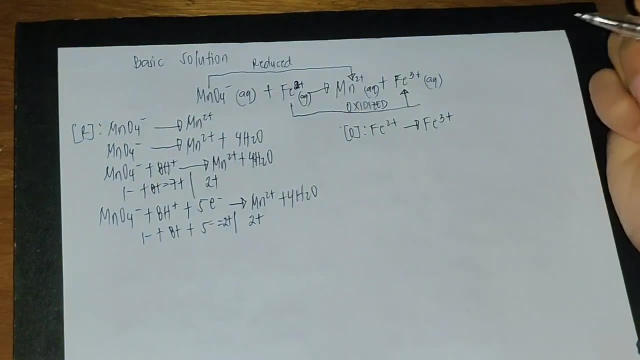 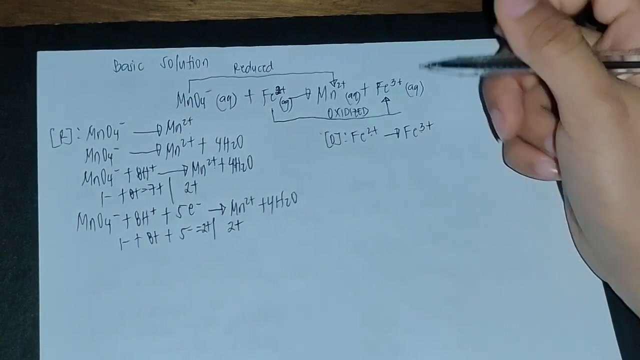 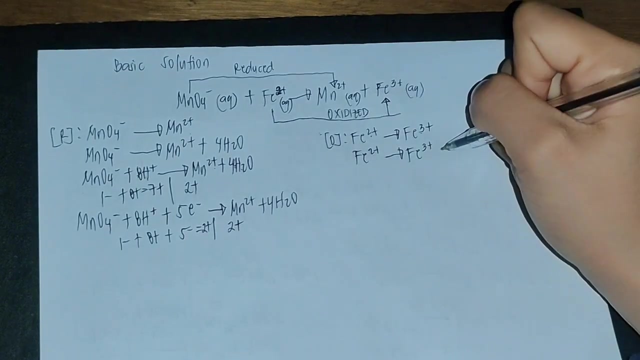 So we move on on the other side, the oxidized parts, So Fe2 positive and Fe3 positive. So in here the charges are the ones that are not. So we have, uh, so just copy Fe2 positive and then Fe3 positive plus electron. 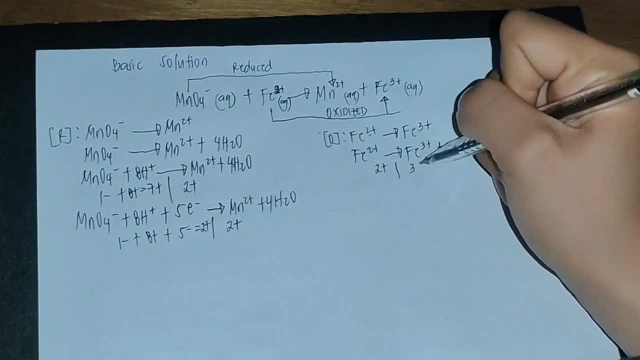 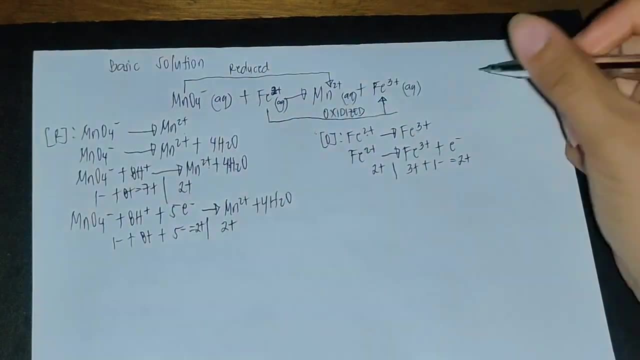 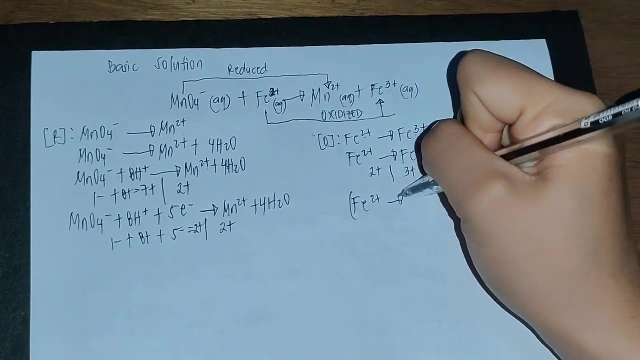 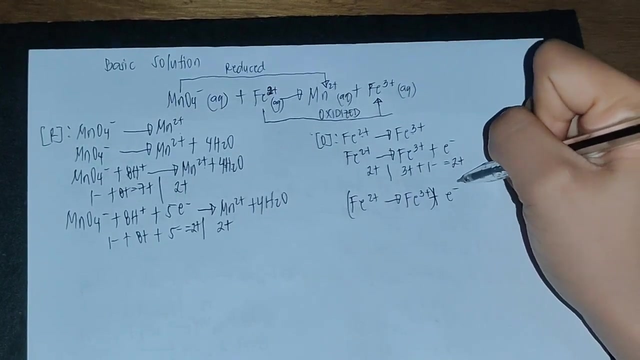 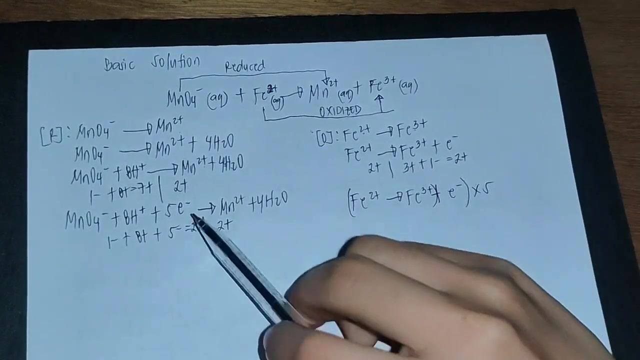 So the charges are now balanced: two positive and on the other side three positive plus one negative equals two positive. So just copy: Fe2 positive and then Fe3 positive times a no plus electron times five. So we need to times the equation with the five so that the electron in the other side will be the same in this side. 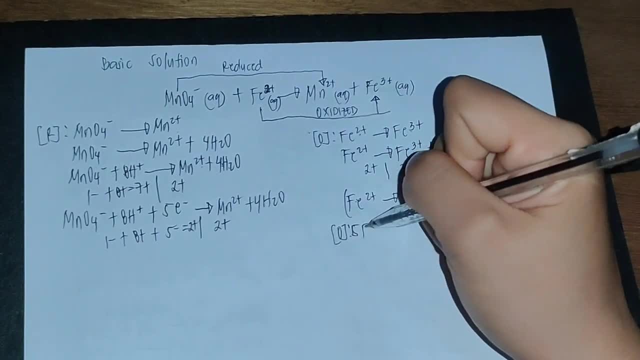 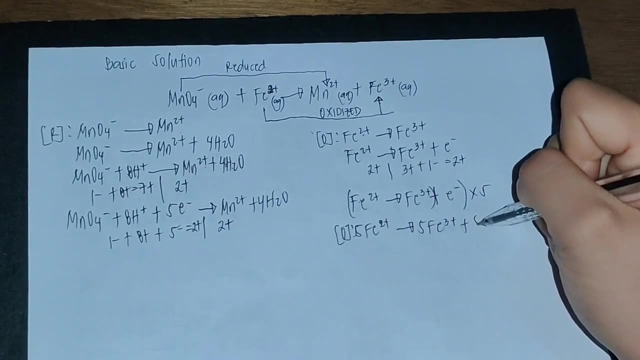 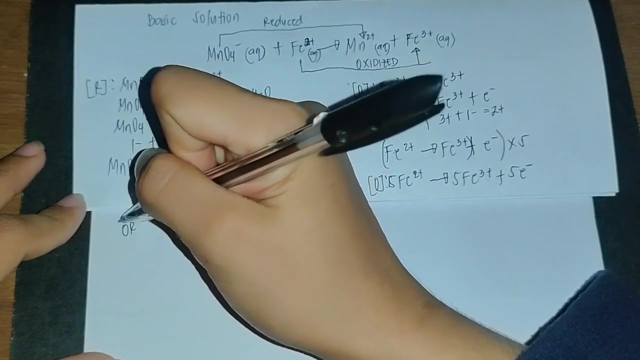 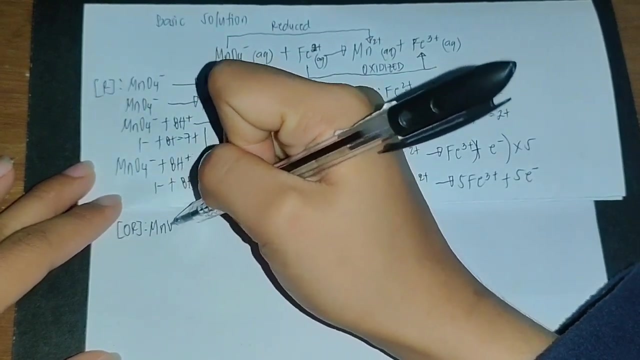 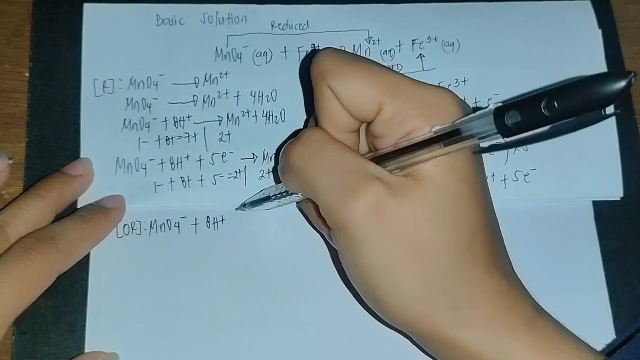 So distribute the five, Five Fe2 plus and then five Fe3 plus Plus five electron. So now we have to combine the two equations. So we write O are here, And then write first the components of the reduced equation. So we have MnO4 negative plus H positive plus five electron, And then 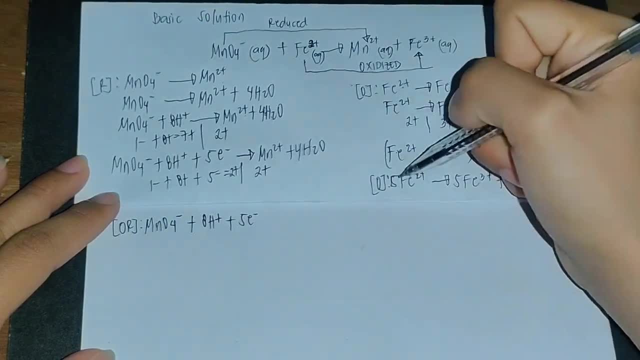 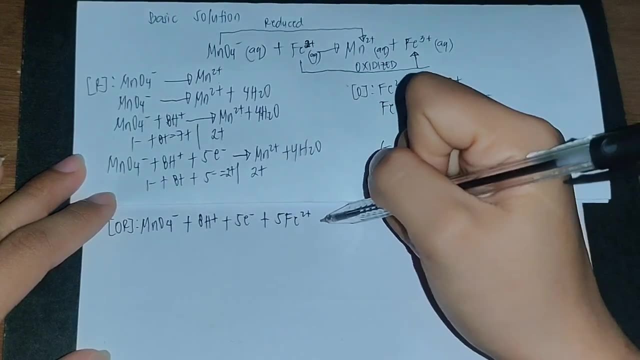 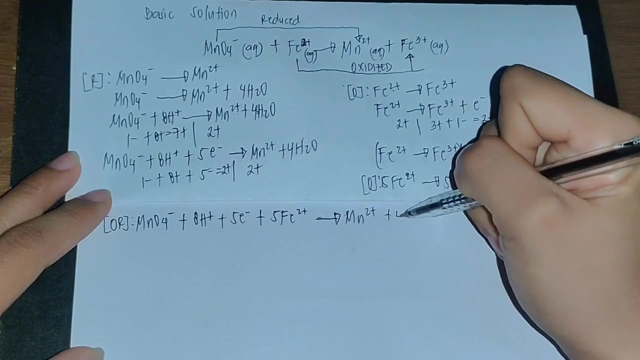 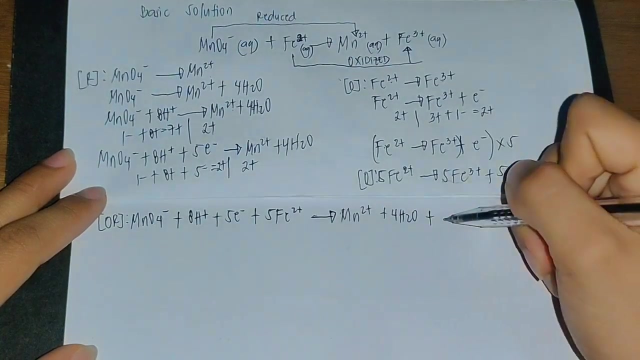 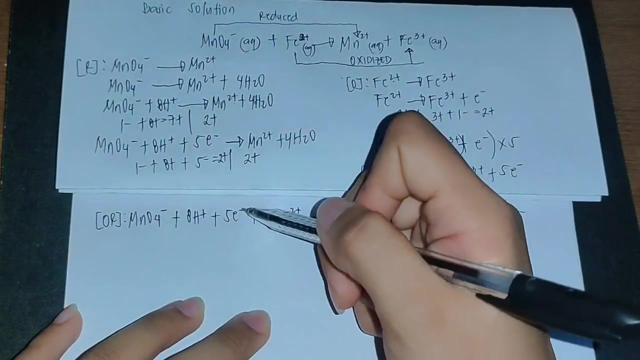 plus 5 electron, And then five Fe5Fe2 positive, and then next is the Mn2 plus plus 4H2O plus 5Fe3 positive plus 5 electron negative. so cancel anything that is the same on the other side, like here: 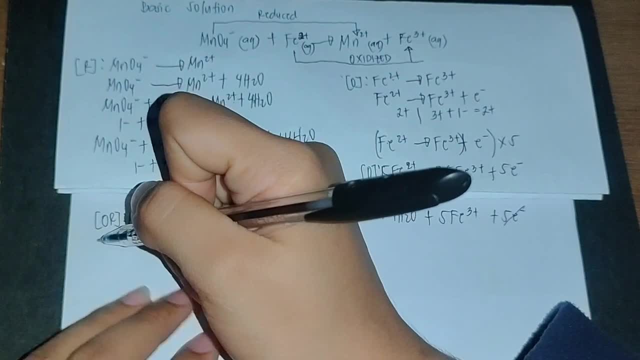 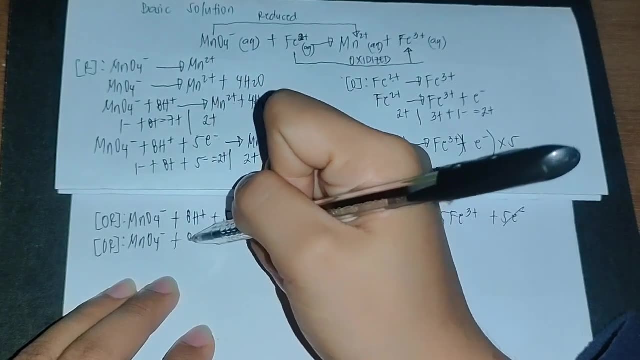 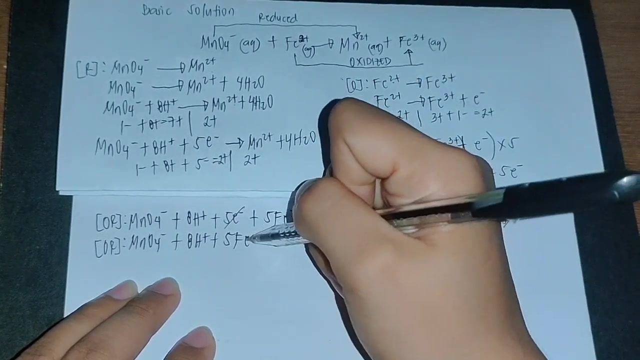 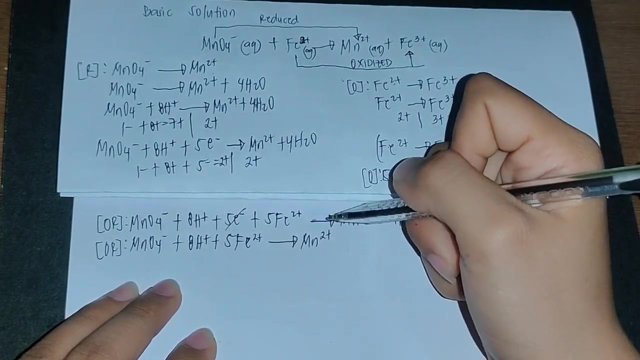 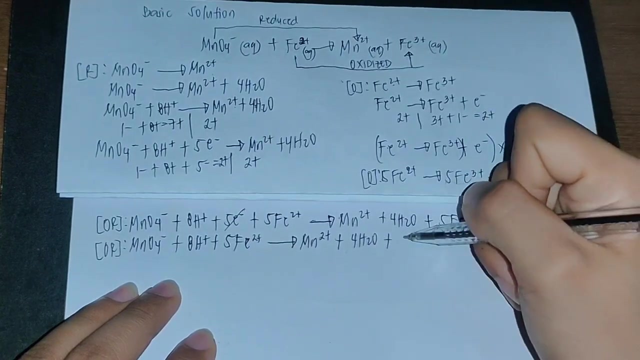 and cancel 5 electron negative. so now we rewrite the final equation: equals MnO4 negative plus 8H plus, plus 5Fe2 plus, and then now Mn2 plus, then plus 4H2O plus 5Fe3 positive. and now we have to check. 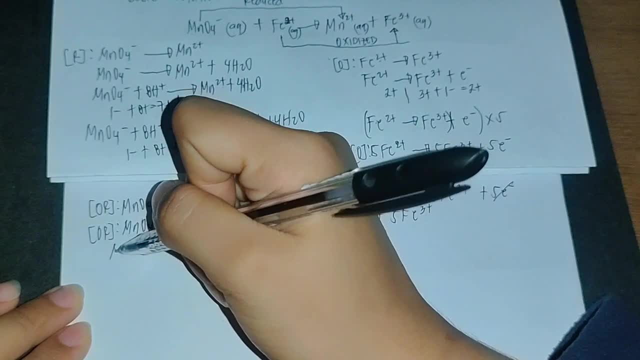 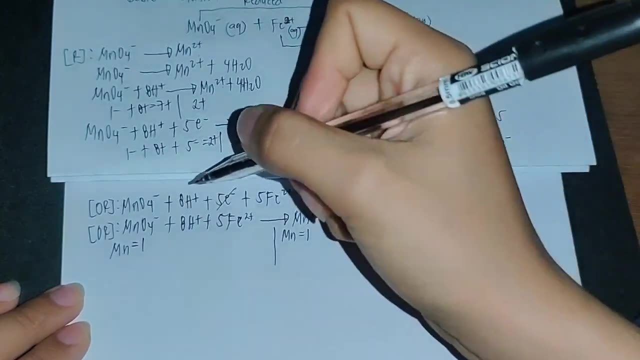 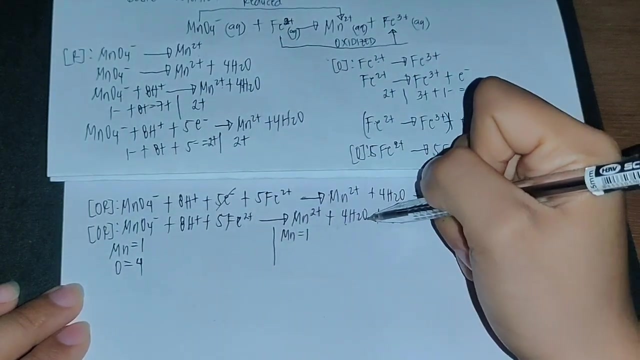 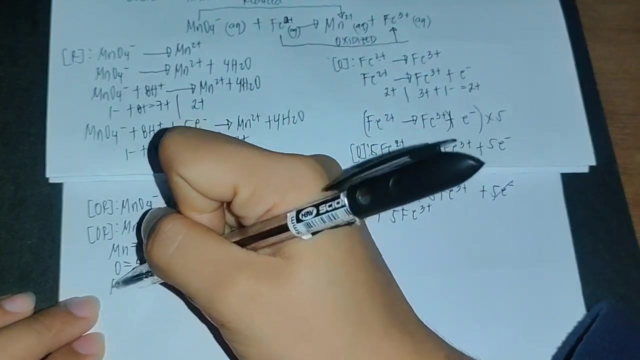 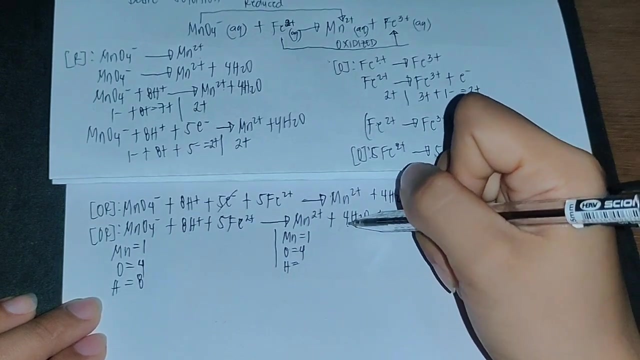 if the atoms are balanced. so Mn- here we have 1, this side we also have 1. and the oxygen, we have 4 oxygen here, we also have 4 number of oxygen here and we have 8 hydrogen here and we also have 8 because 4 times 2. 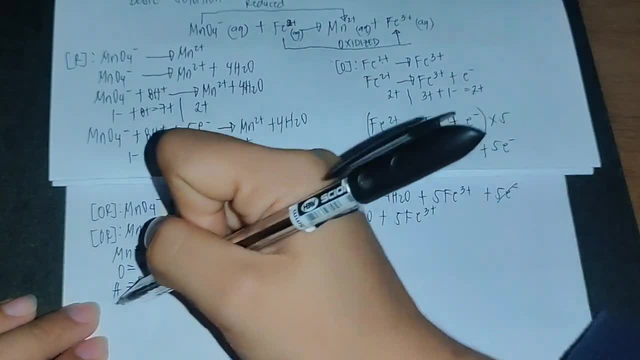 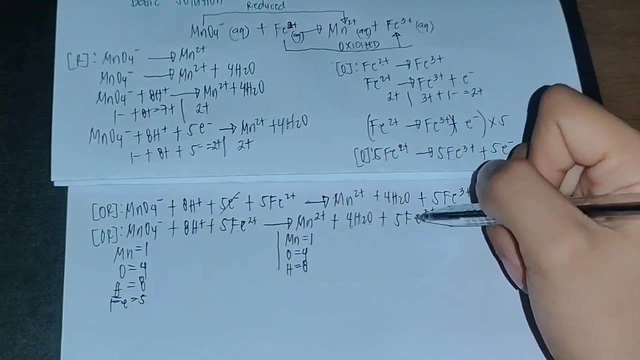 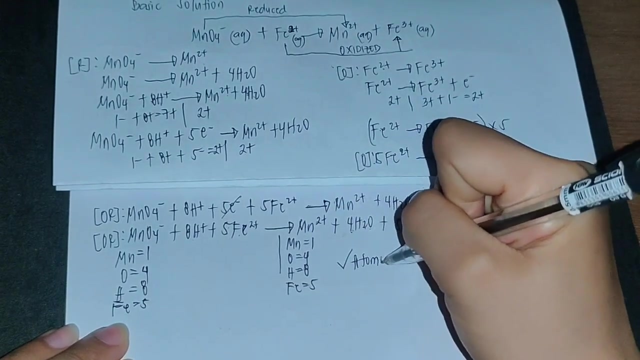 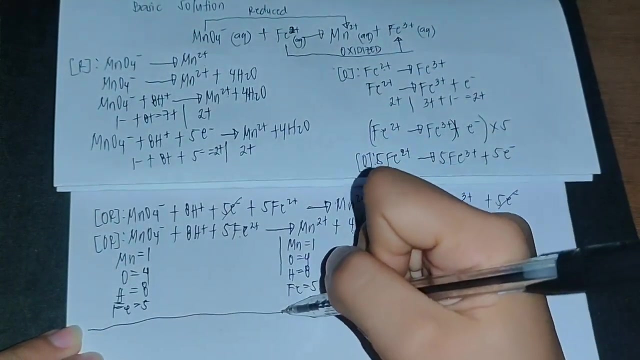 equals 8 hydrogen here. and the iron? we have 5 iron here and on the other side we also have 5 iron and on the other side we have 3 oxygen here. so we conclude that the atoms are now balanced. so next is we have to check if the charges are balanced. 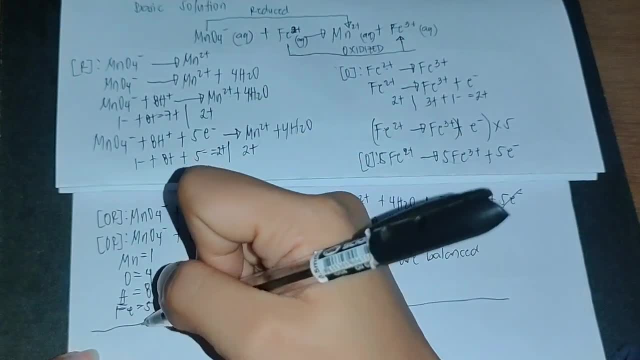 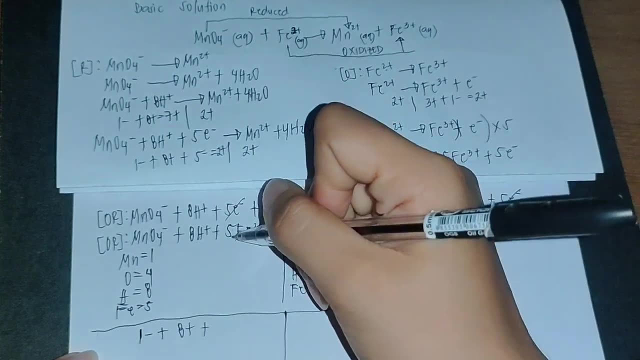 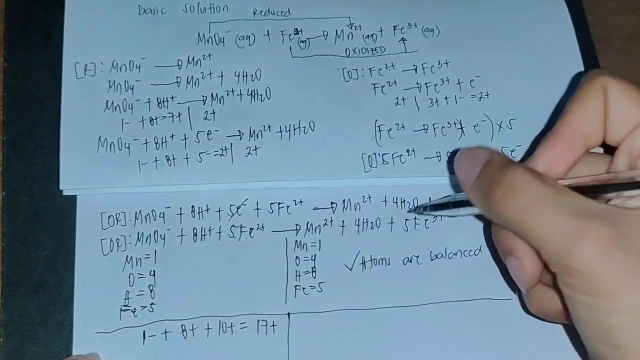 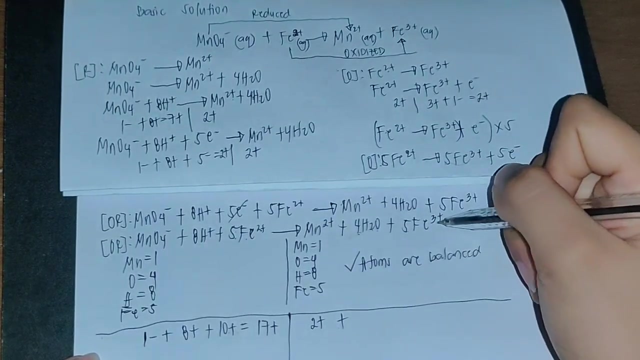 so here we have 1 negative plus 8 positive plus 5 times 2 equals 10 positive, so we have 17 positive. In here we have 2 positive plus 5 times 3 equals 15 positive, So we all have a 17 positive.